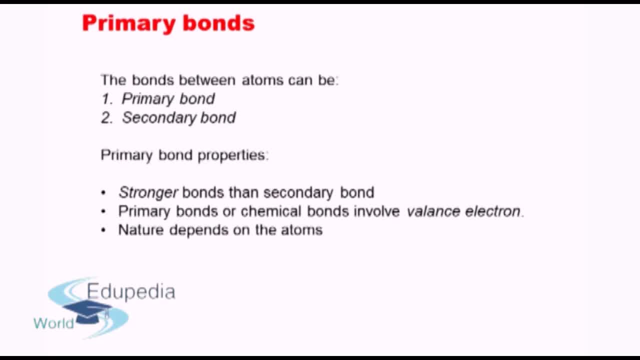 bond. There are multiple types of primary bond. Primary bond will be formed between two atoms will depend on the nature of both the atoms. Now, what are the types of primary bond that are present? Broadly speaking, primary bonds can be divided into three categories. First and foremost, it's called ionic bond. The second 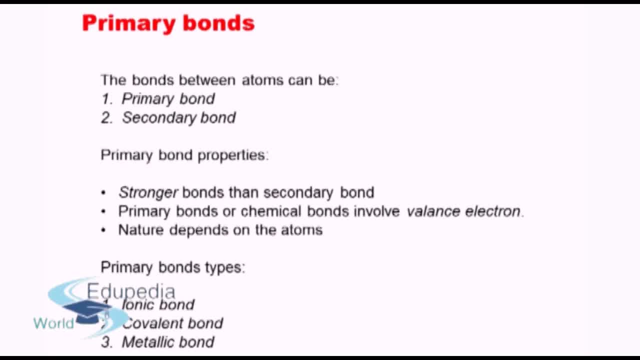 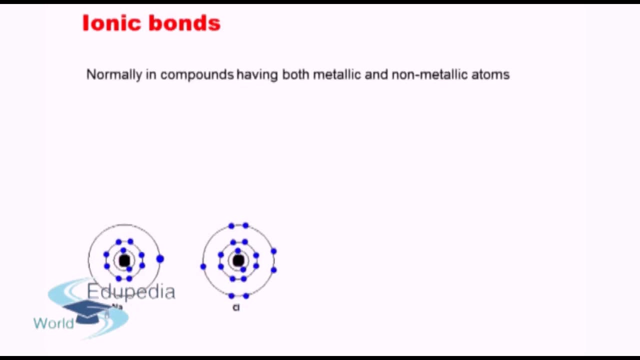 is called covalent bond And, finally, what we have is known as the metallic bond. We will discuss about all three of them in details now Let's start with ionic bond. Ionic bond are the type of bond which normally exist in a compound having one metallic atom. 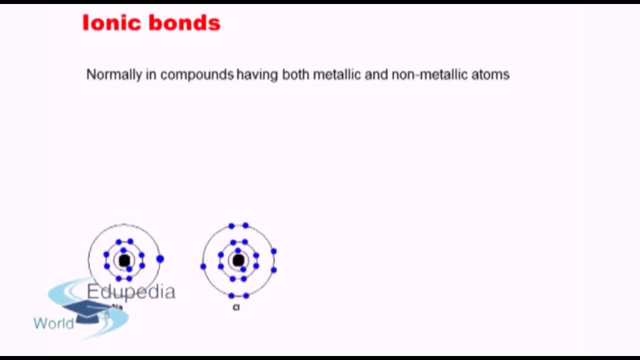 and another non-metallic atom. Put differently, the two atoms participating in an ionic bond generally have large distance of electronegativity. The difference of electronegativity gives rise to ionic bond and the reason as we will discuss now. We will discuss it through an example of sodium and chlorine. Now, you might be knowing that. 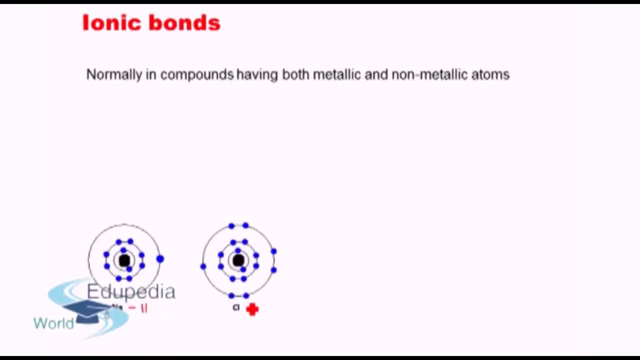 sodium is has 11 electrons and chlorine has 17 electrons. So the configuration is like the first orbit. We will be using the Bohr's model for the simplification, But we can also write 1s2, 2s2, 2p6 and 3s1.. So this gives two electrons and two electrons. So it gives two. electrons and two electrons. So if you look at the first orbit, you will notice that the first orbit is the second orbital- It's the first one, And second one is the second orbital. So the first one is the second orbital. So this gives two orbitals and this is the second. 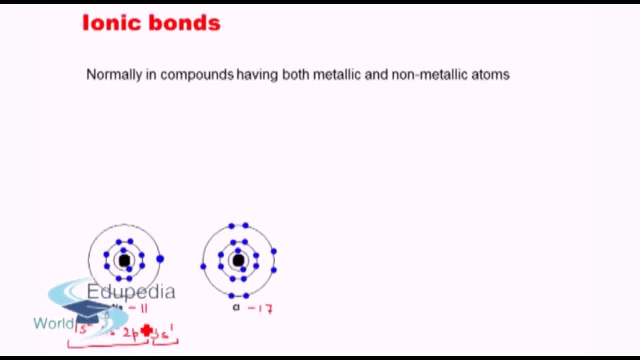 10 electrons, and this is the 11th electron. This 10 electrons lie in the two inner orbit, Only this single electron in the outer shell. Similarly, chlorine has a configuration of 1s2, 2s2, 2p6 and 3s2- 3p5.. Okay, so there are a net of seven electrons in the outermost. 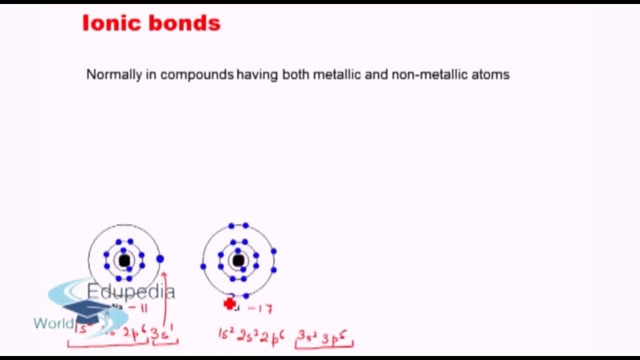 shell. From your basic chemistry understanding, you might be knowing that in order to have a stable configuration, in order to have a noble gas configuration, or the outermost orbit should have eight electrons in it for stability. Now, how can these two atoms attain stability? 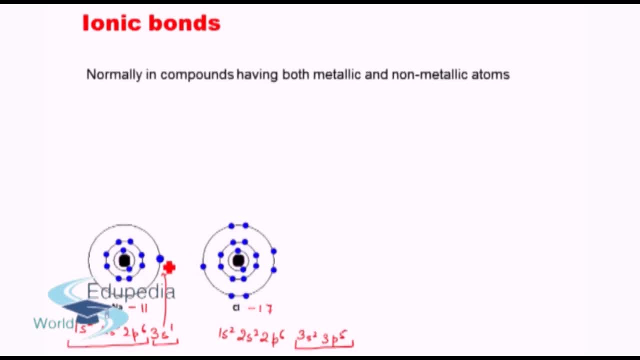 Let's suppose that the single electron in sodium atom here is transferred to the outer orbit of the chlorine atom. What will that give? That will give rise to eight electrons here and eight electrons here, because this orbit no longer exists. This orbit will have eight electrons and the stable configuration will: 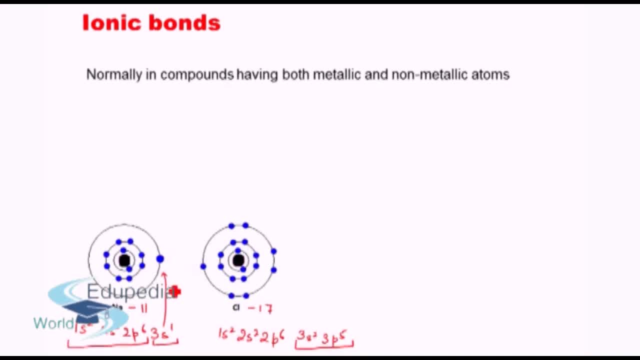 be attained. That is exactly what happens. So the electron is donated by the metal to the non-metal, and that gives rise to something known as sodium chloride, in which, since sodium has lost an electron, it becomes singly positive charged and chlorine, since it gained an electron. 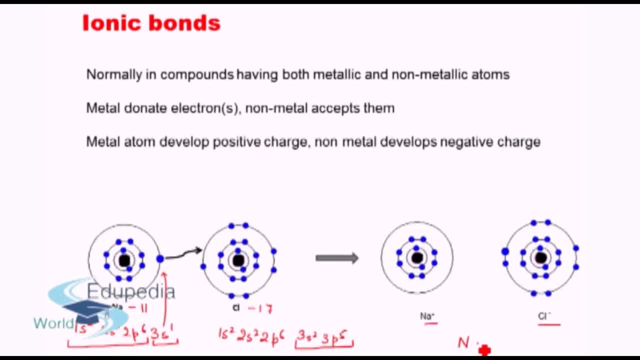 it became a single negative charge and the compound which we got is sodium chloride. This kind of bond that is developed by transfer of electron from one atom to another is known as an ionic bond. This helps attain the noble gas configuration, as I said. Now what are? 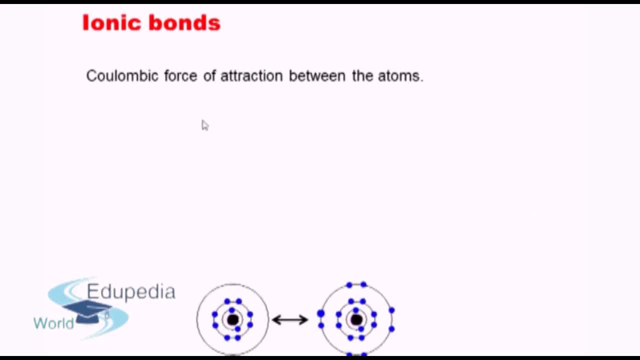 the properties of an ionic bond. There is coulombic force of attraction between the atoms. Why so? Because there is a positive charge here and a negative charge here. There is electrical attraction between the two atoms now and that binds the two atoms together. It is non-directional in nature. What we mean. 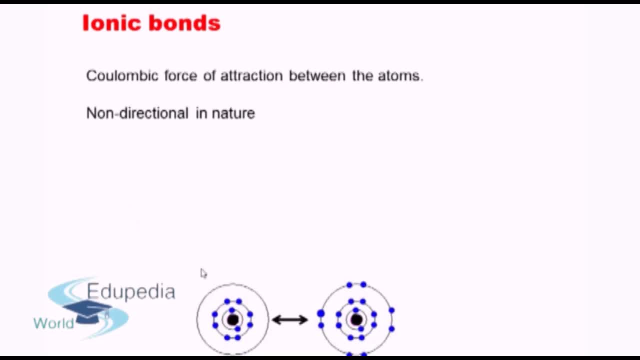 by non-directional nature of an ionic bond is that it does not matter if we have a sodium positively charged atom here. The chlorine atom can be anywhere around here, because charge which spreads its attraction in a spherically symmetric manner, There is no fixed direction. 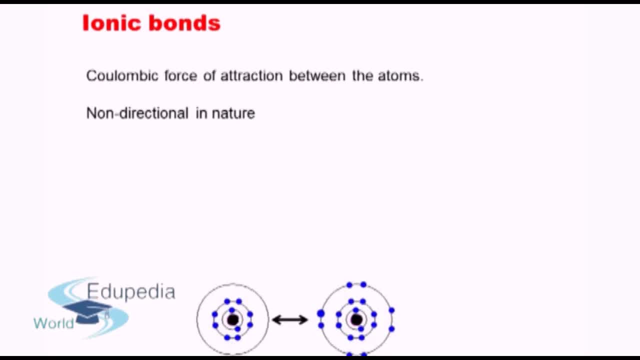 in which it attracts more. It attracts in all the directions similarly, So it is non-directional in nature, As we will see in our discussion about covalent bond. covalent bond is a directional nature bond. That is not the case of ionic bond. The bond energy is relatively large. 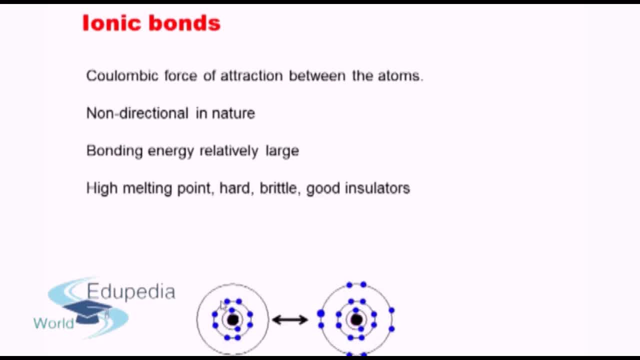 in ionic bonds And this large ionic bond is a covalent bond. This covalent bond is a covalent bond. This large bonding energy results in a higher melting point for ionic systems. Also, ionic bonds normally gives rise to hard, brittle and good insulators, Hard materials and brittle because 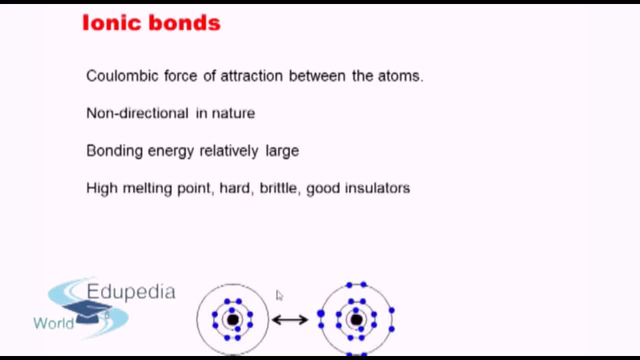 of the strong bond Good insulators, because there are no free electrons, Isn't it? And also the charged particles. the atoms are charged, but they are bound together. Thereby they are electrically neutral. Thereby they are good insulators, Thereby they are good. 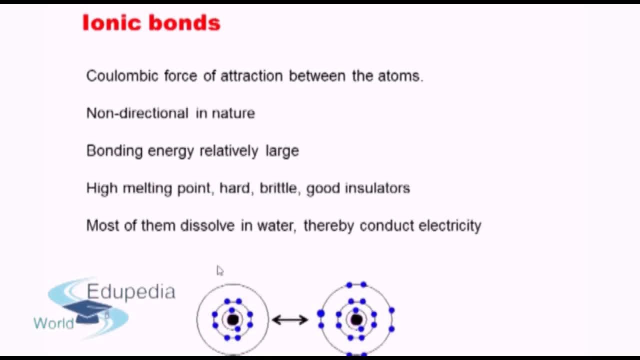 insulators: Ceramic materials. if this, let's say sodium chloride, dissolves in something, dissolves in water: a polar material. this being polar, it will dissolve in water. Thereby we will have charged distribution. There will be sodium plus ion and chlorine minus ion. 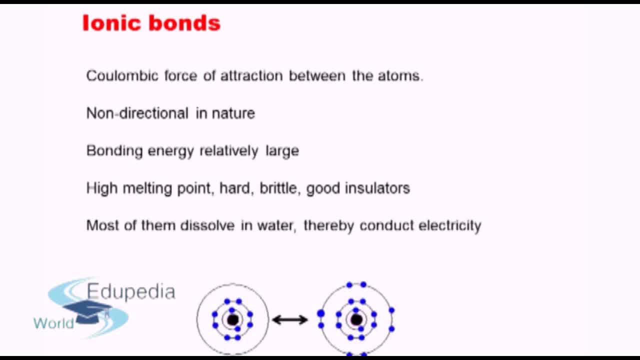 And that will result in conductivity. So the ionic material, when not dissolved in water, are good insulators, But once it dissolves it starts to conduct electrons, and ceramics mainly have ionic bond. This gives you a holistic picture about what ionic bonds are. 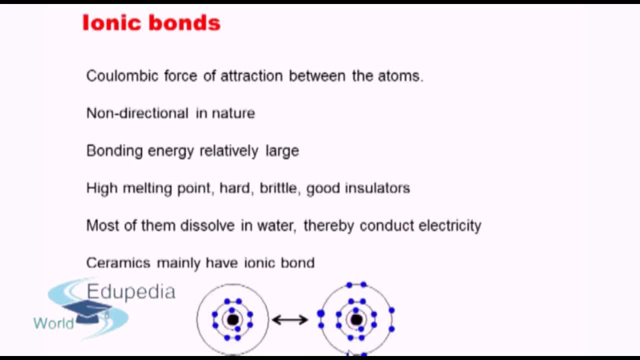 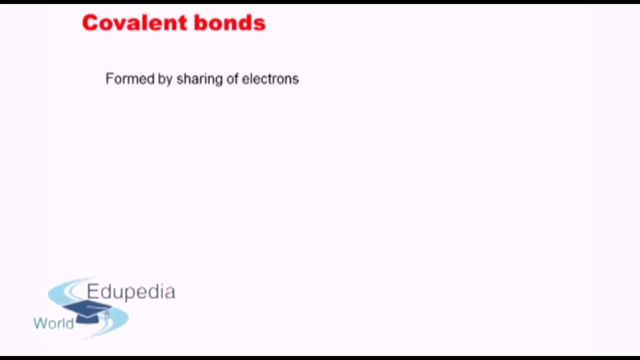 Next let us see the second kind of primary bond, that is, the covalent bond. Covalent bond are formed by sharing of electrons. Ionic bonds were formed by either accepting electron or donating electron. That is a major point of difference between the two. 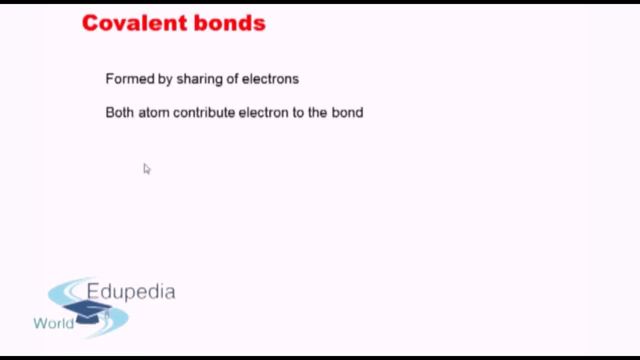 Then both atoms contribute electron to the bond. Since there is sharing, both participating atoms will contribute electron to it. Let's take an example in which now we have both atoms as chlorine Now, since this chlorine atom has seven electrons at the outermost shell. similarly, this has 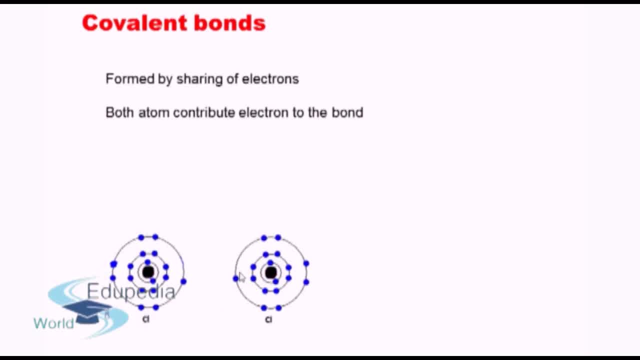 seven electrons in the outermost shell. There is no way one is going to transfer an atom to the other. since then it will become further six electrons. A alternative atom is a covalent bond. The alternative which they find out is that if they share one electron into a common bank, 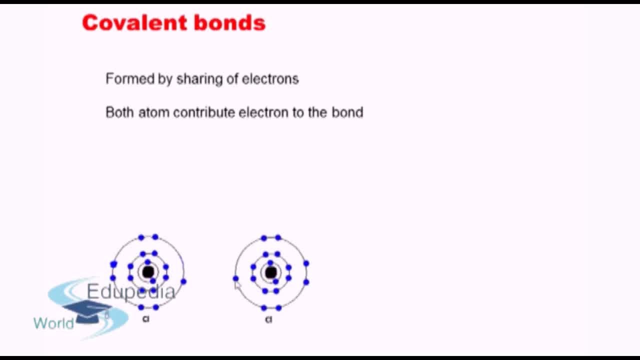 let's say, then both of them will have eight electrons and they will get their stable configuration. That is exactly what the chlorine atoms does. Now, these two electrons are the shared electrons, and these two shared electrons form a single covalent bond. If there were an atom like oxygen, which had six electrons in the outermost shell, 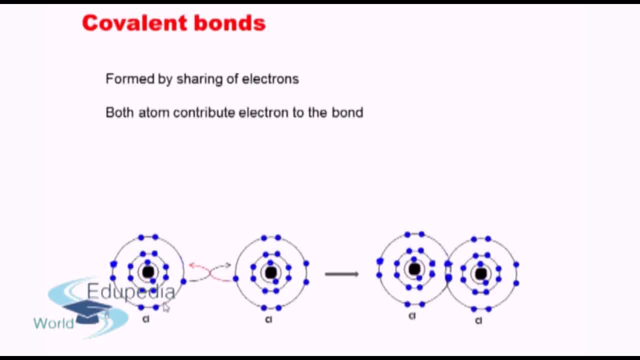 Then each of them would have shared two electrons and we would get four electrons shared effectively. thereby, two bonds will be formed, two covalent bonds. We understand now how the sharing happens And, as I said in the previous discussion about ionic bond, ionic bonds are non-directional. 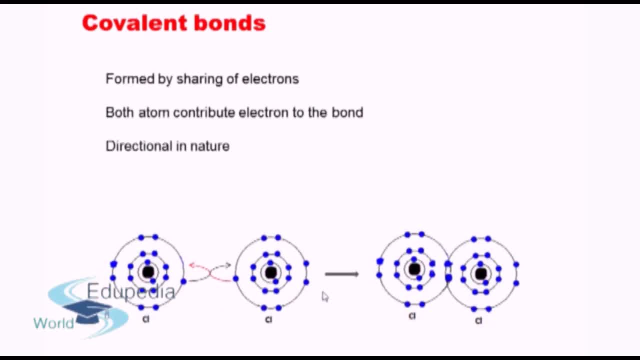 in nature, but covalent bonds are directional in nature. Why so? Because they have sharing of electrons. The electrons lie in between the two atoms. Thereby they are covalent. That is why they are covalent. They are bounded in the 3D space. 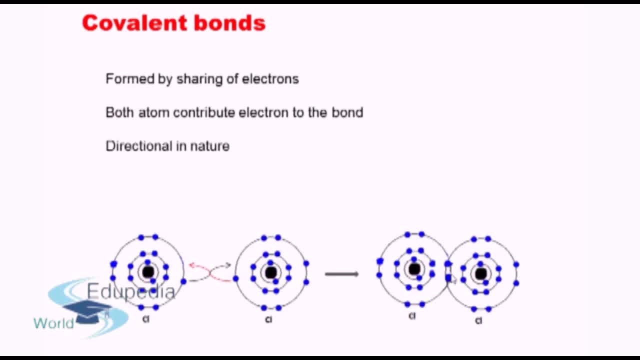 They cannot be at any dangle they want right. In this case, since there are just two atoms, they will always be at 180 degrees, since they are symmetric. In the case of water, where we have H2O1, oxygen, 2 hydrogen, there is an angle, something like. 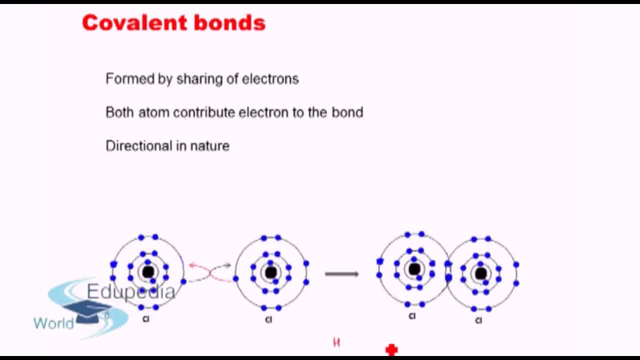 this: Oxygen here, hydrogen, here The two. hydrogen shares one electron, The oxygen shares one electron each and the oxygen shares two. thereby oxygen has another four. So it completes its octet. The only exception to the octet rule is for hydrogen, where it can take two and form novel. 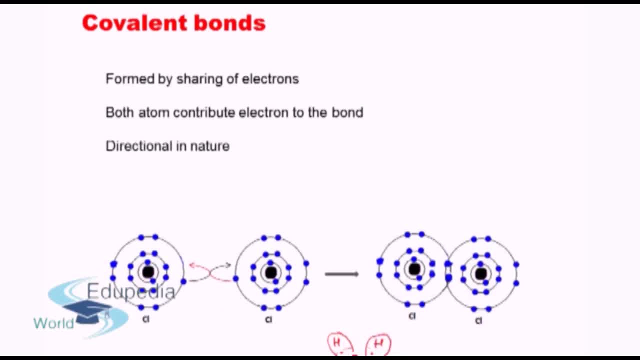 gas configuration, the helium configuration. Therefore, we can see here that the angle in which the two hydrogen can be with respect to the oxygen is defined by the H2O1. The, And we can see in this case the covalent coulomb of the two atoms, from hydrogen to H2O1, for 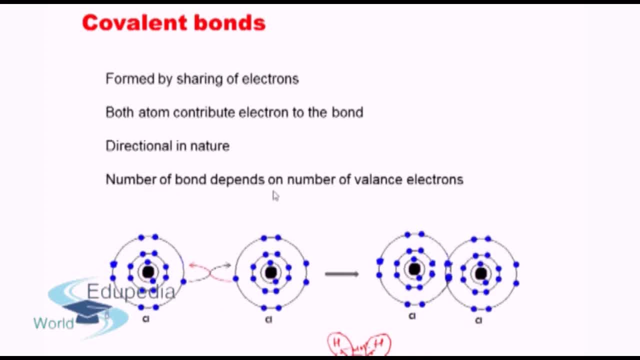 nitrogen. Now when do we start to learn about the covalent bonds? The first thing we need to know is the bonding nature, And this is roughly 109 degree for water. That is what we mean when we say that covalent bonds are directional in nature. 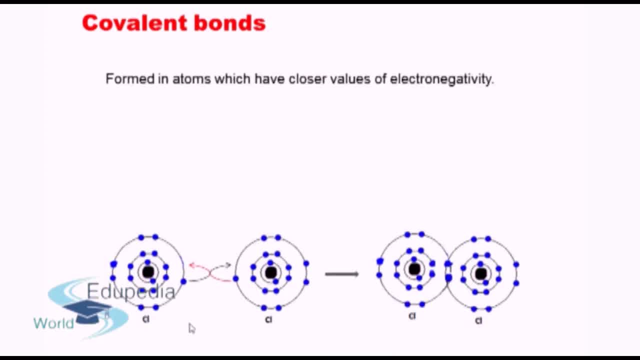 Number of bonds depend on the number of valence electrons. As I discussed, for chlorine we will have single bond, For oxygen we have to have two bonds And for nitrogen three bonds. Now, when is the covalent bond formed? It is normally formed when the two participating atoms have closer values of electricity. 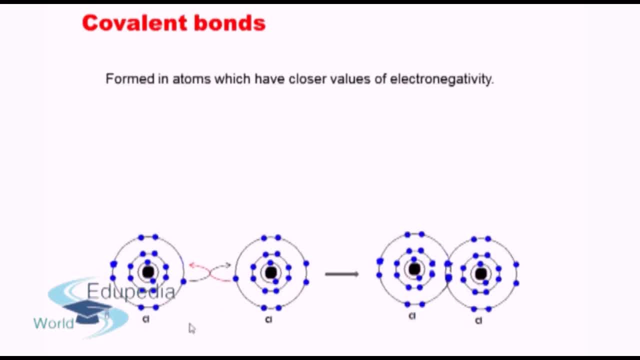 values of electronegativity for ionic bond, the two participating atoms had a huge difference electronegativity. covalent bonds should have closer electronegativity. thereby they should be willing to share electrons, and this is a important point that, though, we have discussed as if ionic 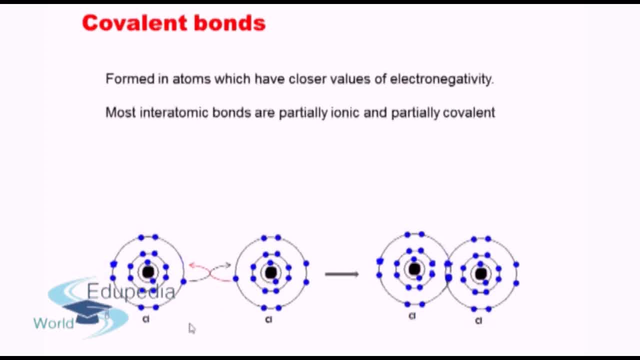 nature exists independent of covalent nature, or covalent nature and ionic nature cannot coexist. but in reality, since there is at least some electronegativity difference between most of the atom, except for the cases when both are same atom, then there is no 100 percent covalent or no. 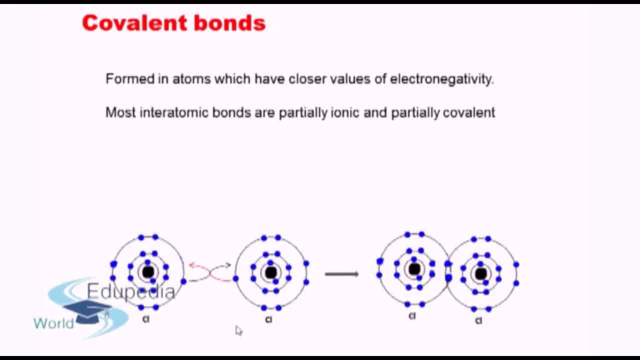 100 percent ionic bonds- rather they are partially ionic or partially covalent- may be more covalent if they are closer in electronegativity, more ionic if they are further in electronegativity. that is for the covalent. 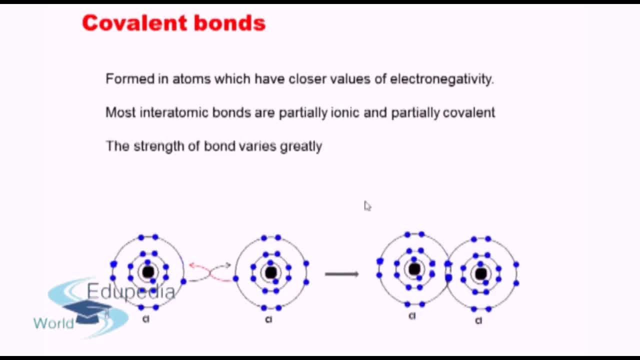 bond nature, the strength of the bond really varies. it can be very strong bond in a covalent bond or it can be a very weak bond, like in this example. bismuth has a very low melting point because its bond strength is quite weak, whereas diamond has a very, very high melting point because 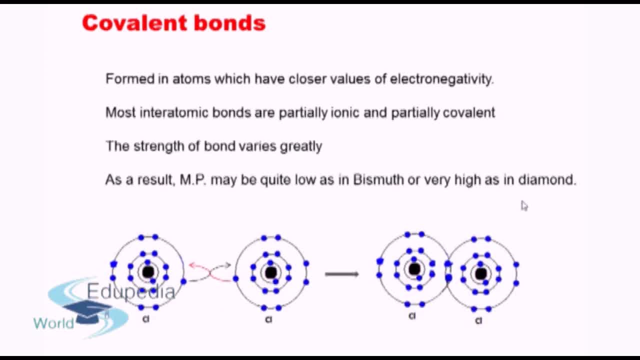 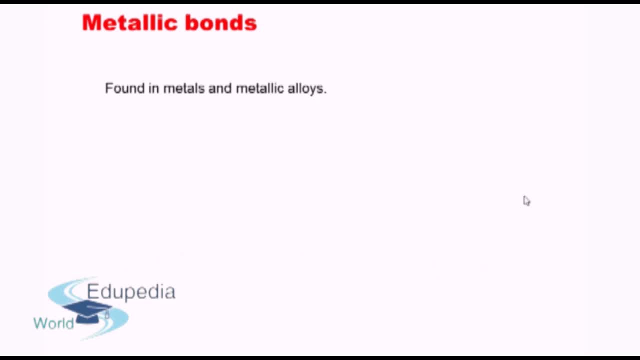 it has one of the strongest covalent bond known to mankind. now let us discuss the third kind of primary bond, that is, metallic bond. metallic bond are formed in metals or metallic alloy systems. we know that in the metals normally only one, two or three electrons exist in the outermost shell, so it is not possible for them to share electrons and gain the. 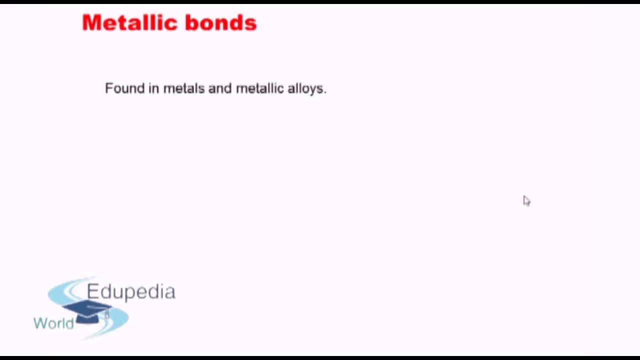 octet stability. nor is it possible for them to transfer electrons and gain octet stability. so instead, what they do is that they shear electron to the whole bulk and thereby attain octet stability at the atomic level. so if we have a single, let's say sodium or some metal, it what it will do it will. 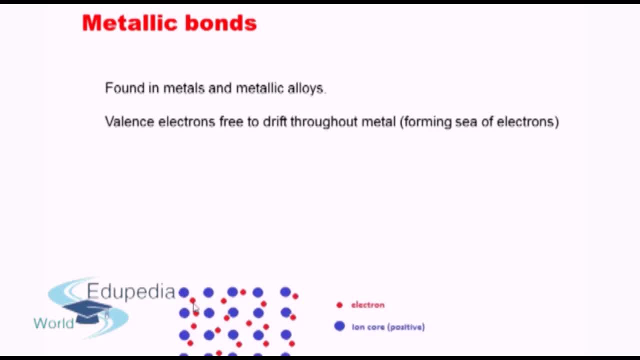 have a ionic core which will remain positive, and the electrons become part of a large sea of electrons drifting throughout the metal. that is how the metallic bond is formed and again here the bonding nature is non-directional. metallic bonds similar to ionic bond are non-directional and the bond energy and the melting point varies greatly. as we know, metals 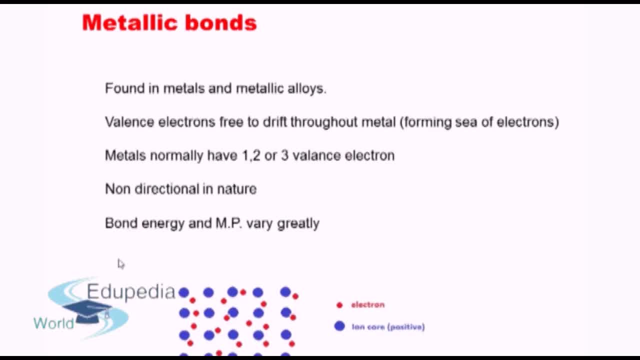 like mercury, are liquid at room temperature, whereas other metals, like tungsten, has a very, very, very high melting point. you cannot pinpoint that metallic bonds are always strong or always weak. this gives you a rough idea about the third kind of primary bond. to briefly summarize, we have 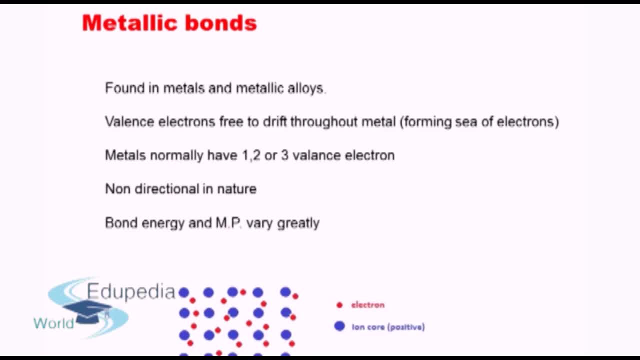 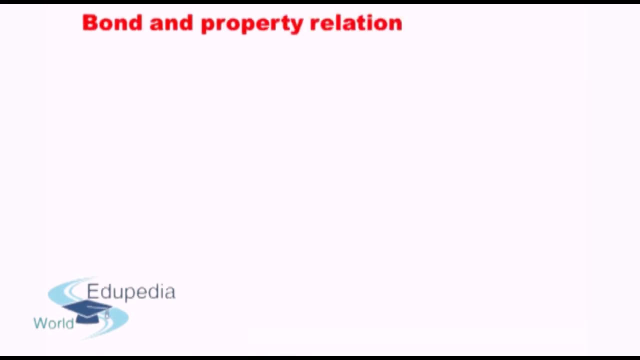 three kinds of primary bond: ionic bond, which is formed by transfer of electron from one atom to another. covalent bond, which is formed by sharing of electrons. and metallic bond, which are in metal systems, by giving up its valence electrons in the sea of electron. what are the bond and property? 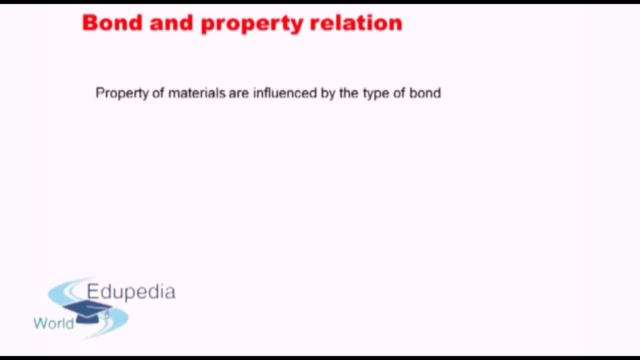 relations. the property of a material is highly influenced by the type of bond, as we saw that something which has a strong bond will find it very difficult to be in the molten state. a lot of energy will be required to melt it. so let us discuss the bond. 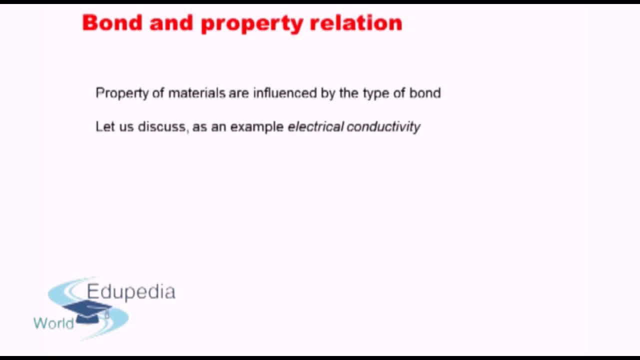 property relation. using one simple example of electrical conductivity, covalent bonds, covalent materials, are insulator. why so? because they have no free electrons available. this is a generic statement. there may be cases where covalent bonds are electrical conductive conducting, but generally speaking, covalent materials are insulated. 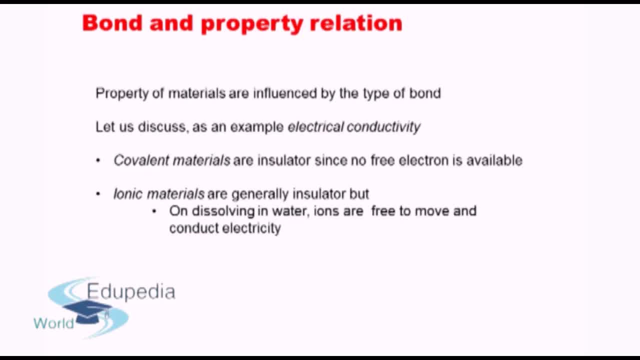 so we see that covalent bonds are very good insulators. ionic materials are generally insulators, again, because there are no free electrons. but when you dissolve some ionic material in water, then ions will be formed, separate out and that can conduct electricity and finally metallic materials. 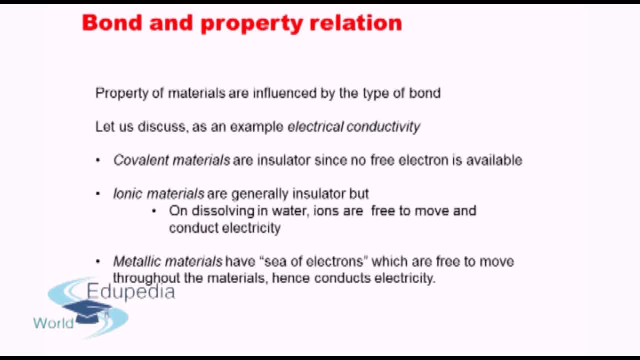 normally they have a sea of electrons which are free to move throughout the body of the material. thereby they are very, very good conductors of electricity. so therefore, with the which갠 to bond the bond, so we can understand the nature of the bond, how we can understand what property it should have, and also if we see a material and have a property. 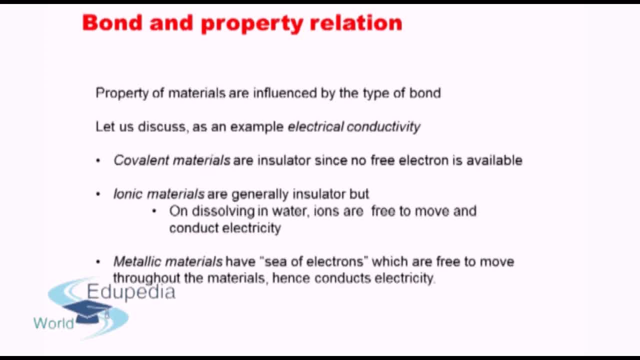 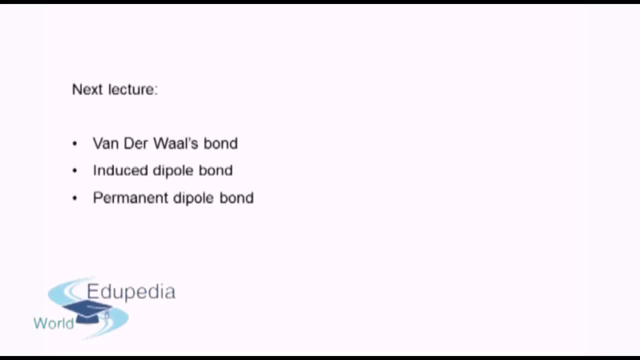 of it we can derive back what kind of bonding it has. this brings us to a conclusion on our discussion about the different kind of primary bonds. next lecture will focus on the different kind of secondary bonds, about van der Waal bond, induced dipole bond and permanent dipole bond. Hopefully you got a good 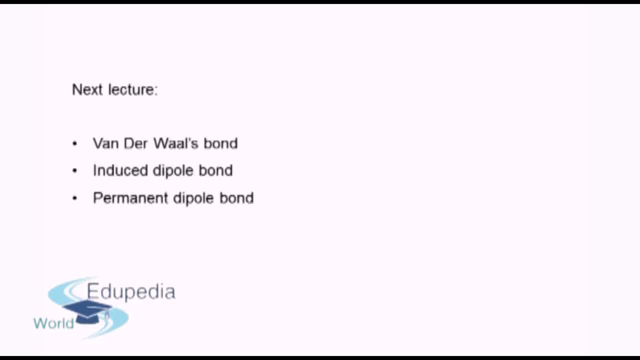 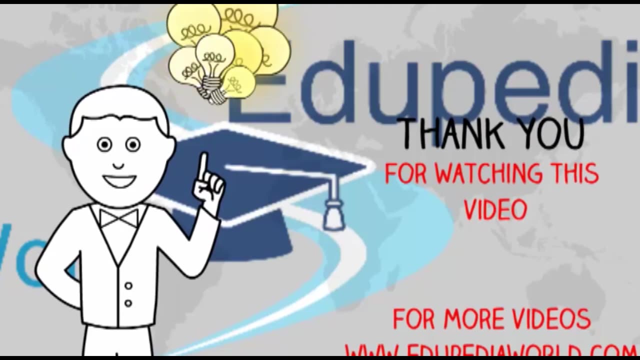 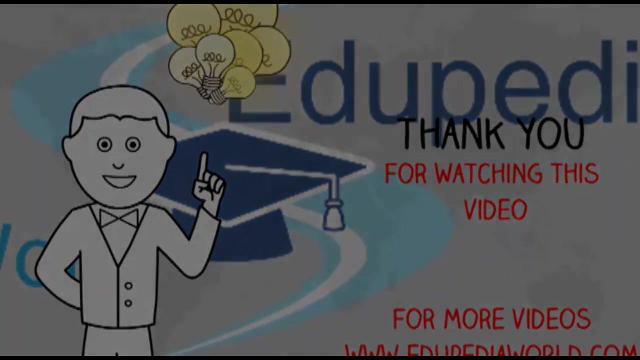 grip about different kinds of primary bonds, and hoping to see you in the next lecture to understand about secondary bond. Till then, have a great day, Goodbye.